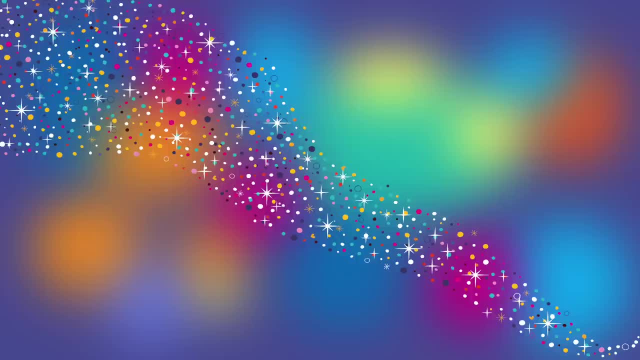 You can breathe and blink as normal, Just see if you can keep your body nice and still Your eyes are open. Now that you're still, can you notice your breathing. Maybe you can feel it a little bit In your chest, Maybe your tummy. 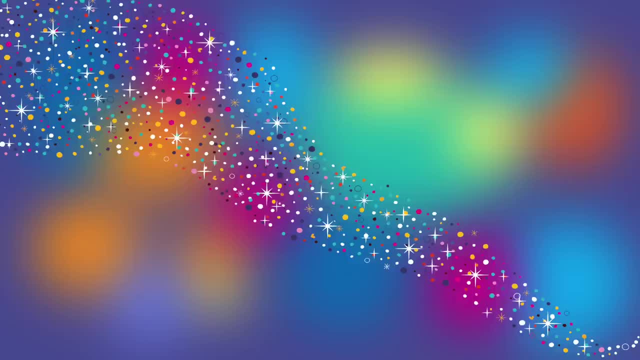 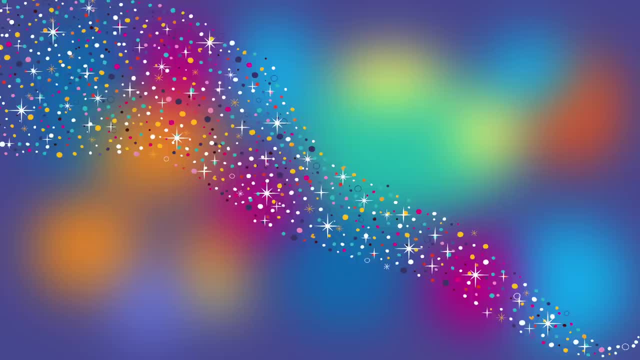 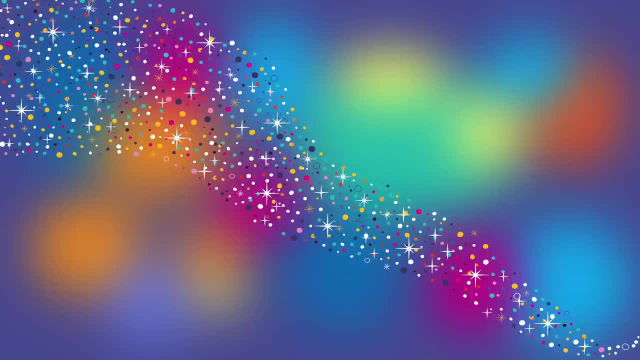 That's it. That's it, Gentle breaths Coming in through your nose and out through your mouth. In through your nose and out through your mouth. This next time, as you breathe out, Let your eyelids softly close. Well done. 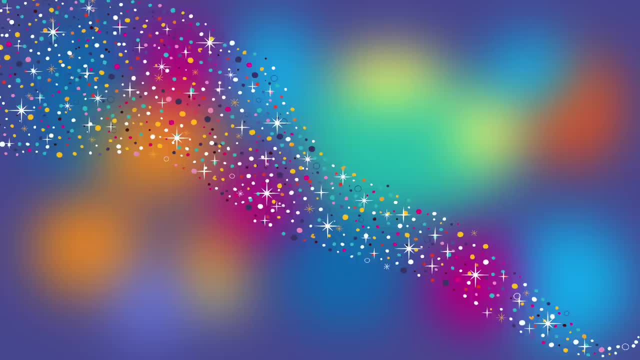 Now, Now, Now You have a big blank screen in your mind. See if you can imagine a little pixie standing right in the middle of it. That's right, a pixie, A small, fairy-like creature. Think about how it looks. 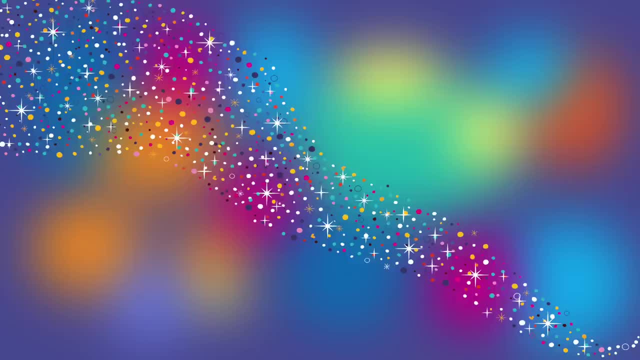 Does it have wings? What colour are its eyes? What's it wearing? It may be a girl pixie or a boy pixie or an animal pixie. You decide how your pixie looks. One important thing, though, is that this is a friendly pixie. 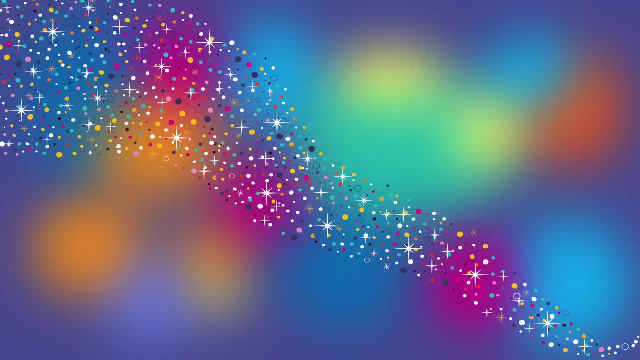 It's a good one. This pixie loves using pixie dust for tickling. Not the kind of wriggling, giggling and jiggling tickles, Just a light, fuzzy tickle. That kind of feels nice and relaxing. 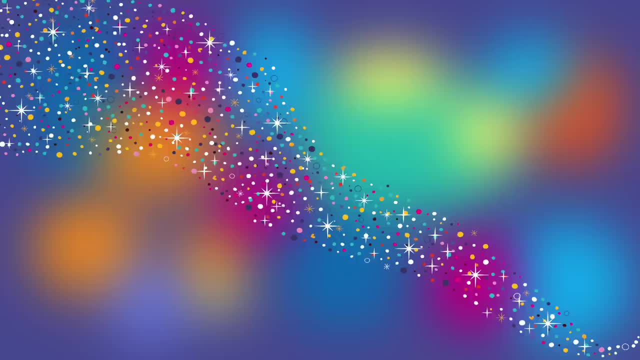 The tickle pixie sprinkles magic pixie dust on our body And we feel it because of the slight tickling. It's a lovely feeling that happens where it's been sprinkled. Let's see if we can notice the feeling when the tickle pixie sprinkles the magic pixie dust on us. 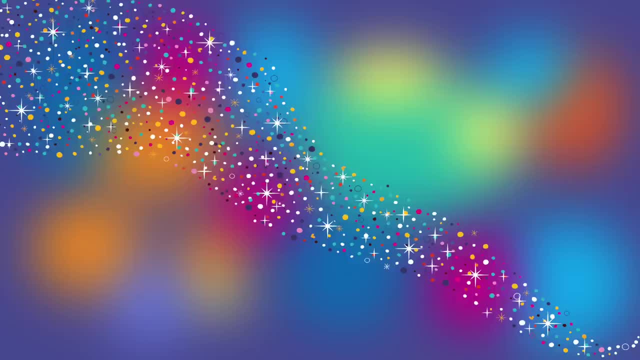 Ready. OK, Let's be as still as we can and see if we can feel the little tickles. Here we go. The tickle pixie starts by sprinkling our feet. There's already a little tingle in our toes, Can you feel it? 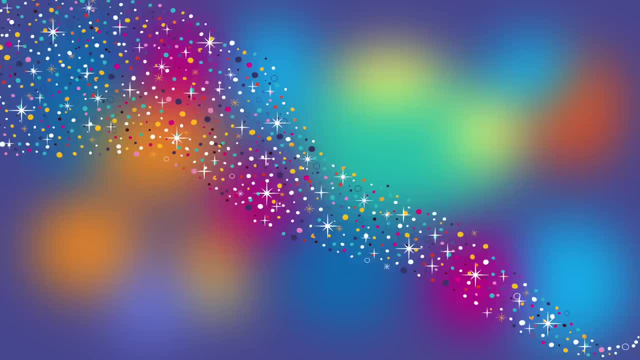 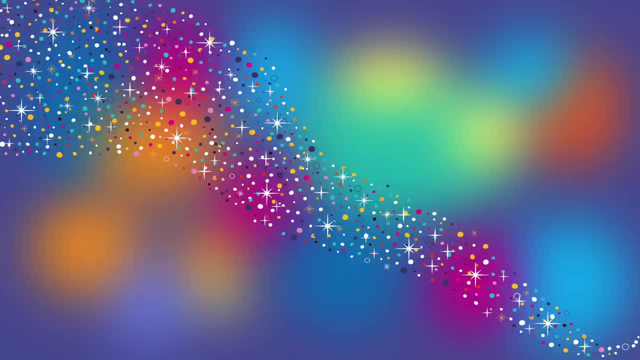 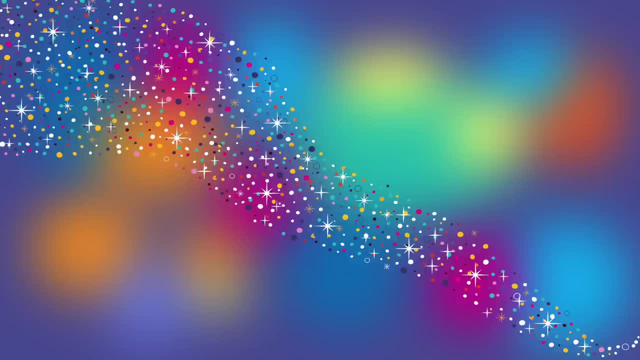 They feel all warm and sparkly. We begin to smile as we notice the tickly feelings. Now the pixie sprinkles the magic tickle dust over the middle of our body, our hips on our tummy and up across our chest. 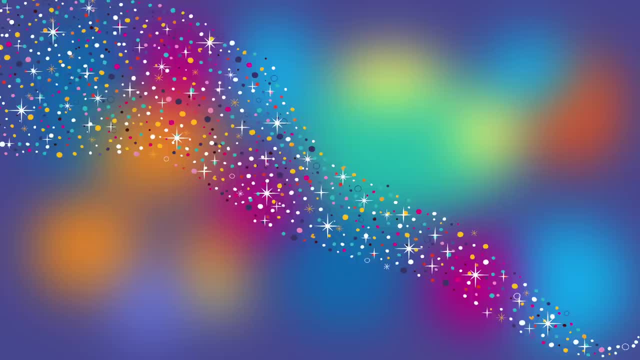 Our body feels the fuzzy tickles, like we are full of twinkle lights. The tickle pixie carries on with the sprinkling. Now we feel the tickles travel all the way down our arms, right to the very ends of our fingertips. 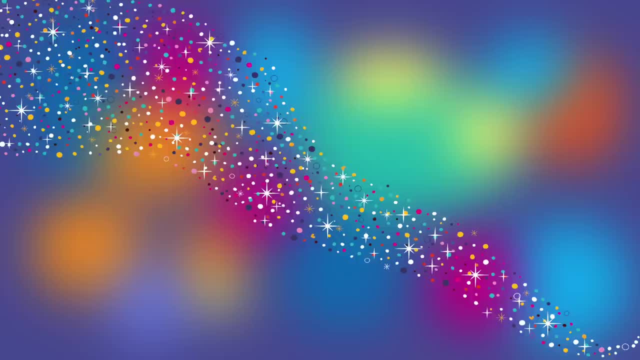 And now coming back up our arms again and over our shoulders. Now the fizzy feeling tingles through our neck and up into our head. We feel our face tingle with the tickly dust. It may even make our nose wrinkle. Wow, what a magic feeling. our whole body is tingling with sparkling, tickle pixie dust. 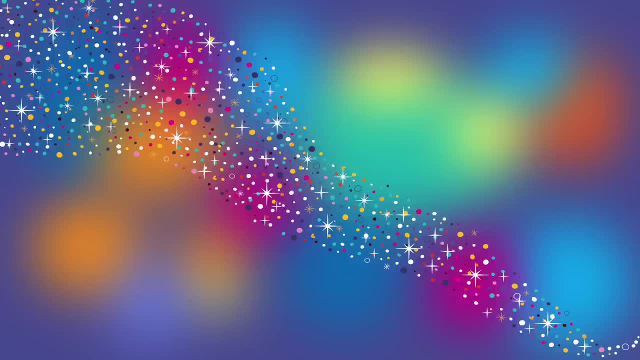 We feel fizzy and sparkly all over The tickle pixie has done its job. You see it in your mind, smile at you and blow you a sparkly pixie dust. kiss, goodbye, Bye, bye. It disappears in a puff of magic dust and the screen in your mind is once again blank. 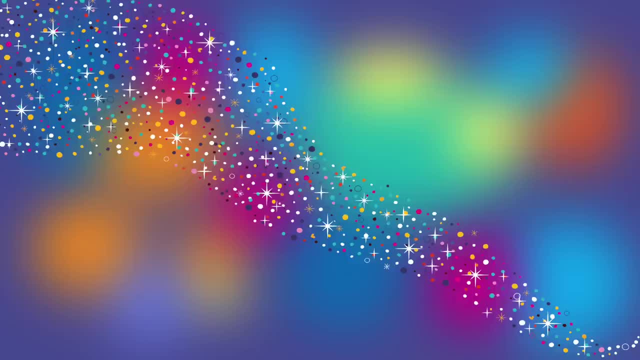 You smile, feeling happy that your body has felt the magic of the pixie dust. And without saying the words, you think a big thank you to your little pixie. And without saying the words, you think a big thank you to your little pixie. 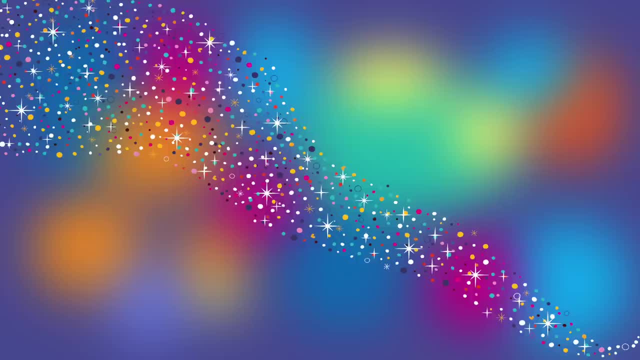 And without saying the words you think, a big thank you to your little pixie. It's time to return now. We come back slowly. See if you can notice the sounds around you. See if you can notice the sounds around you. Feel where your body meets the ground. 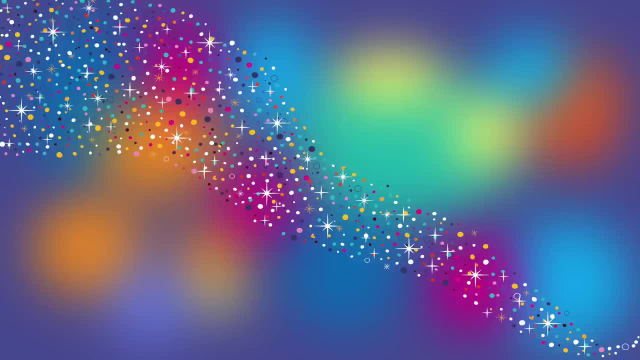 Have a good stretch. Have a good stretch Making your body long like spaghetti. Making your body long like spaghetti. Making your body long like spaghetti. Make your body long like spaghetti, like spaghetti. Take a nice big breath in, Let your stretch relax and sigh out of your 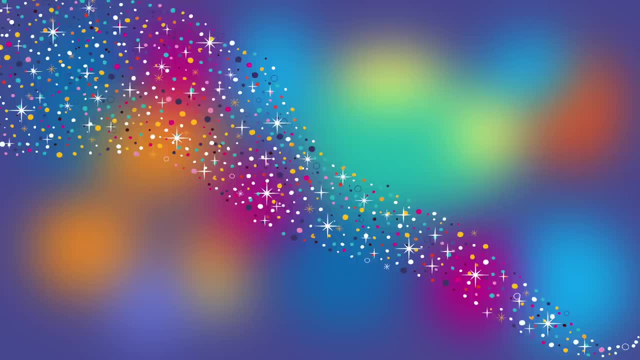 mouth, Gently open your eyes And now just sit or lie where you are for a minute. How was that? Having the pixie dust sprinkled all over you? Maybe you can still feel it a little. Well done for giving yourself this time to stop breathe and feel your body from.